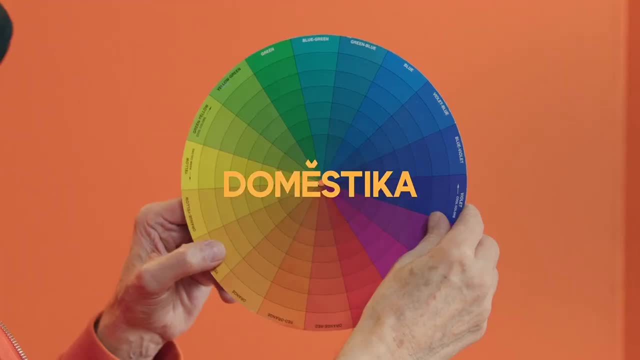 Hi, my name is Richard Mayle and I'm a designer. I'm also an adjunct professor at the School of Visual Arts in New York City. Over the years, I've become an expert in teaching the color experiments invented by Johannes Hitton at the Bauhaus and Joseph Albers at Yale. 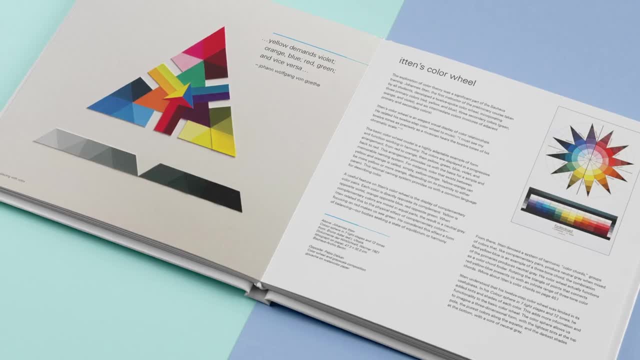 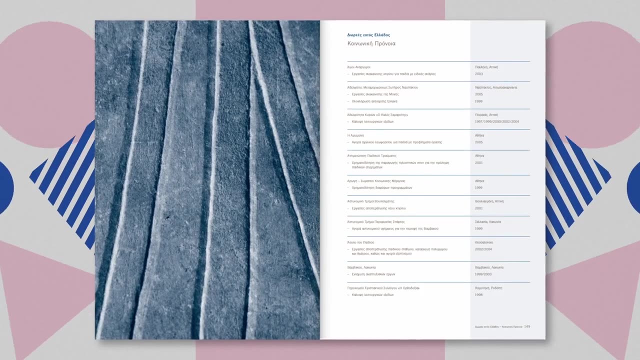 And I'm the author of Playing with Color: 50 Graphic Experiments for Exploring Color Design Principles. I work mainly for institutions and nonprofit organizations, including the Stavros Niarchos Foundation, Leonard Cheshire Disability and the Milken Institute. 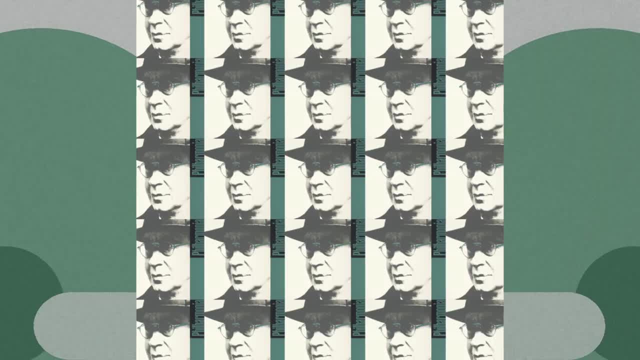 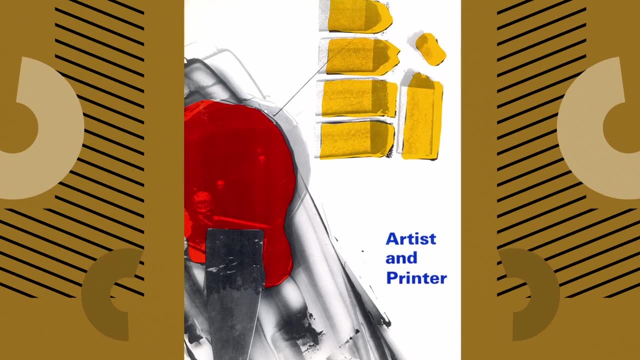 I consider myself a formalist. I love making visual compositions and I feel very lucky to be able to play with forms and the illusions color can create. in both my personal art and my professional practice, I've been taught that to be a good designer, we must first 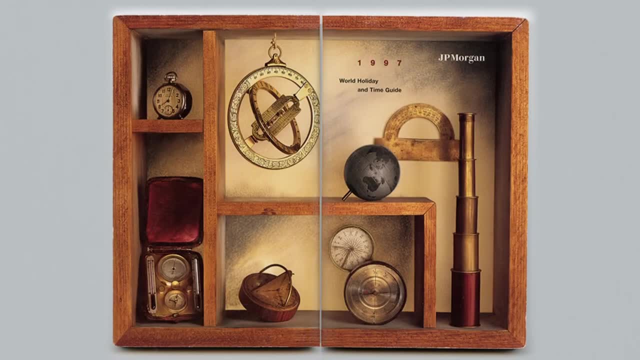 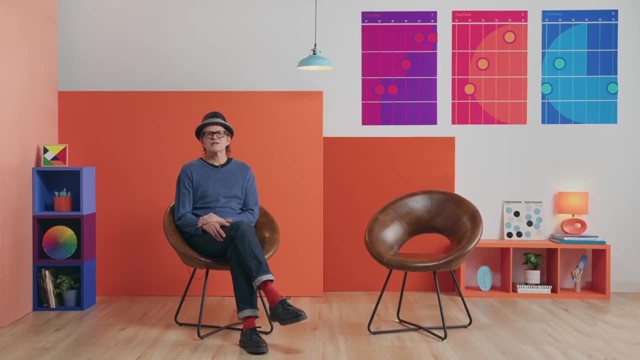 be good artists. Graphic design requires us to use all of our art skills in service to someone or something outside of ourselves. I do my best to live up to this principle. In this Domestika course, you will learn to learn about the relativity of color and practice ways of applying it in graphic. 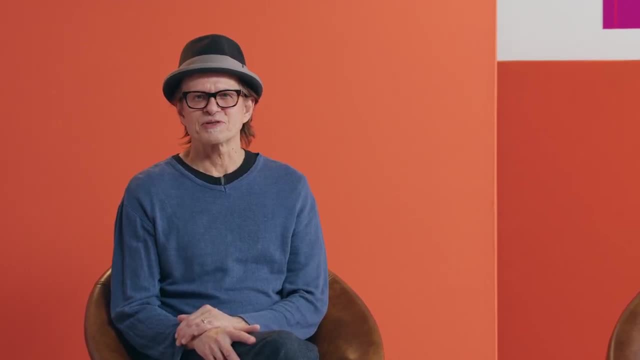 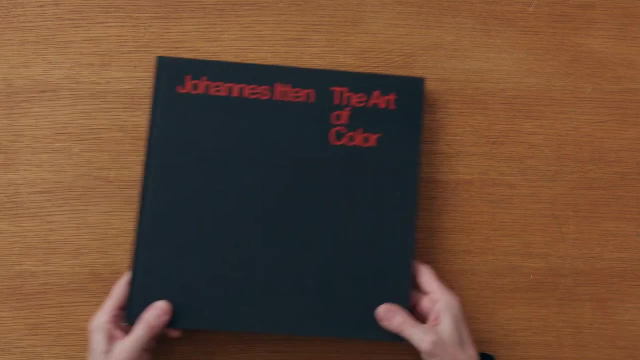 design For the final project. you will create a set of exhibition posters, as well as an animated version of one of them. First, I'll introduce you to Itten and Albers classic books on color theory, and we will experiment with the latter's color subtraction, doing sketches. You will then learn how to create the 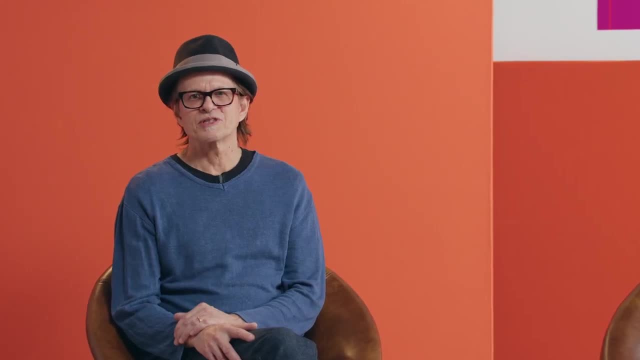 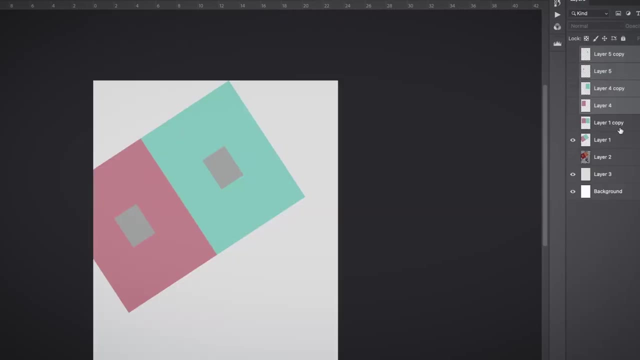 illusion of transparency. After giving you an overview of poster design, I will guide you through the creative process. We'll take our best three colors, look like two sketch and turn it into a full-sized poster in Photoshop. We'll then do the same with our transparency and space illusion design concepts Next. 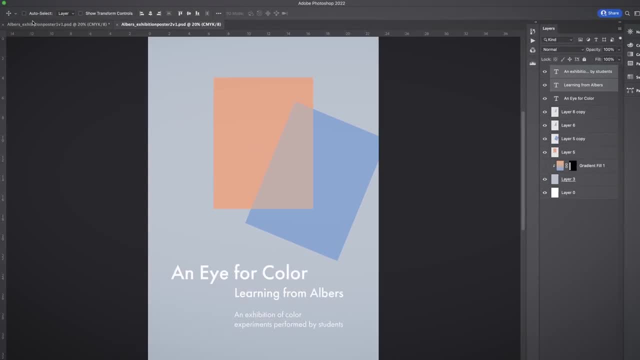 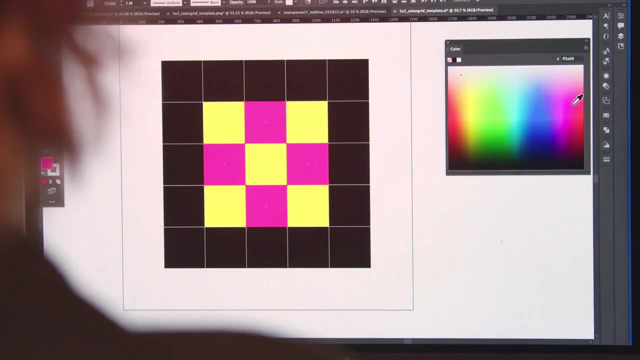 we'll discuss type treatments for posters and develop our own. Lastly, we'll animate our digital posters. By the end of this course, your new knowledge of color principles will make your creative process more engaging and enhance the quality of your design products. You will need drawing material and basic. 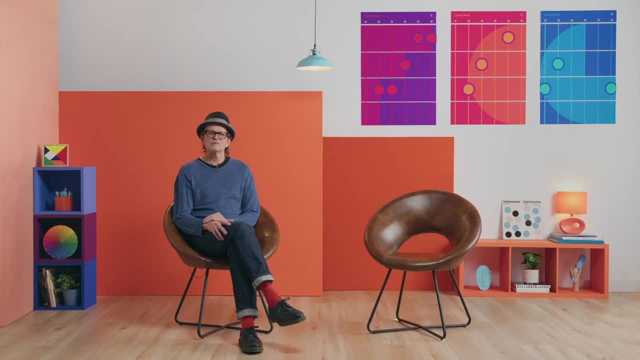 photoshop and illustrator skills. Learn about color. it'll make you a better, more confident designer.